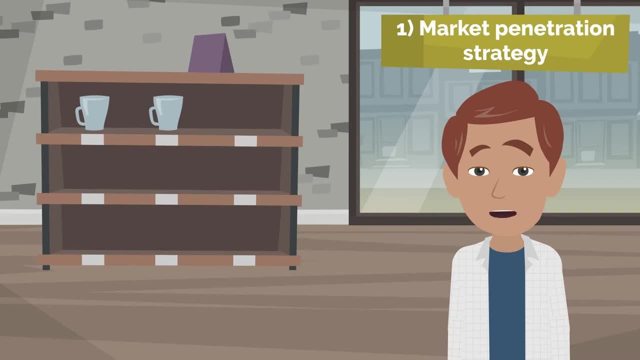 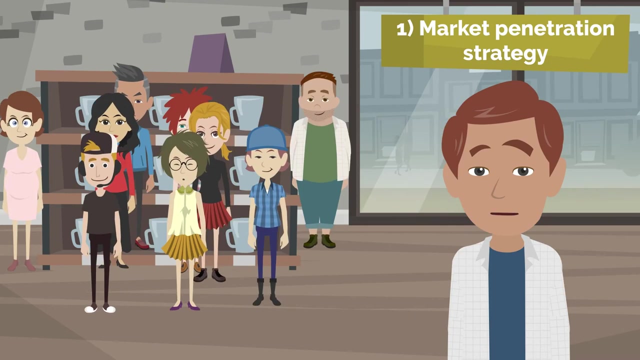 existing market. The market penetration strategy is used when a company can develop on the existing market by offering the products it has at the moment. In this case, sales and promotional activities are most often intensified in order to reach new customers while simultaneously increasing the sale of the goods among the present customers, Sometimes minor, visual. 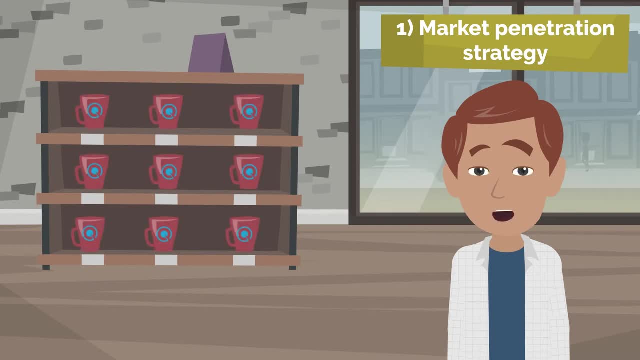 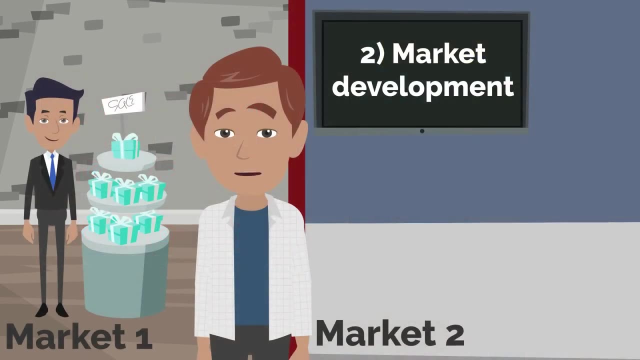 changes are applied to refresh the appearance of products or their packaging without drastic changes in the functions and properties. According to ANSOV, the second possible strategy is the market development. It aims to enter new markets with the existing product. It is used by companies that are unable to increase sales in the markets in which they 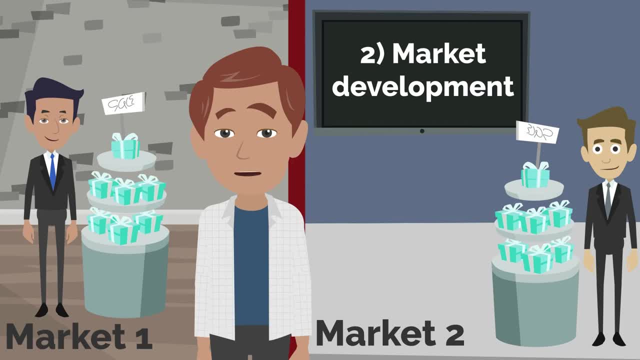 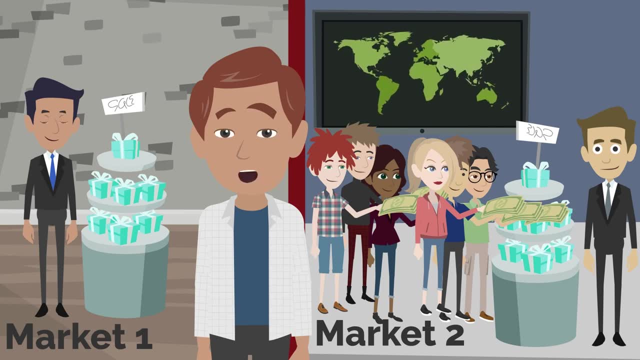 are already present and therefore decide to sell products on a larger scale. In a scenario like this, two forms of expansion are available: A geographic expansion of the market through the introduction of products from the domestic to international markets. In this case, it is necessary to adjust the product range to the specificity and needs of the customers. 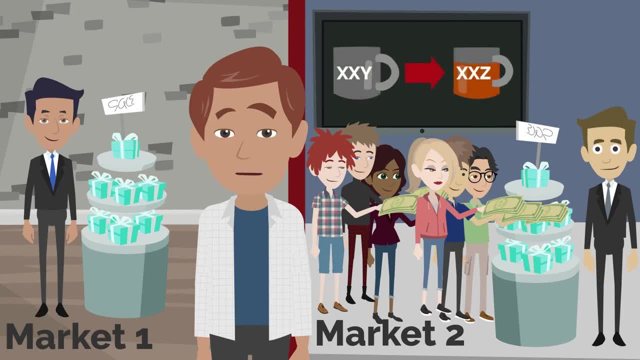 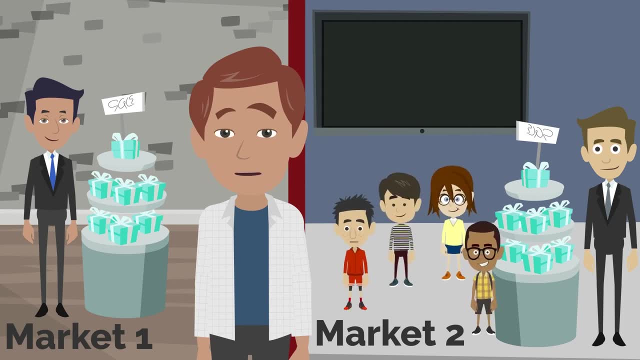 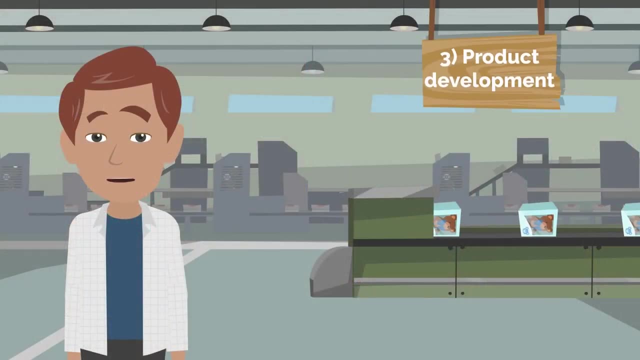 in a specific market, for example, by changing the packaging or name of the product. Another way is to enter new market segments by reaching new target groups through promotional activities and brand repositioning. The third strategy developed by ANSOV is product development. As with the previous strategy, it is used when a product cannot develop further on the 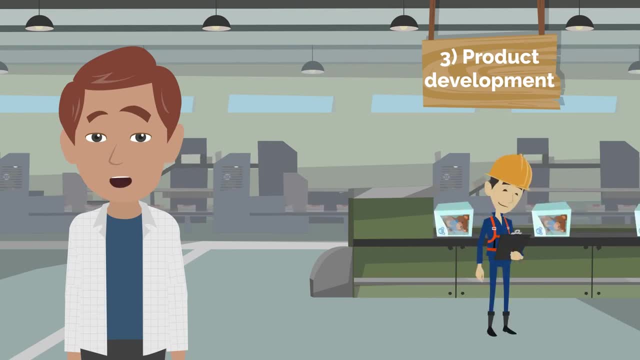 on the current market. This time, however, the strategy assumes that the company will not expand the distribution nor intensify the promotion of its product range, but will work on introducing a completely new or heavily modernized product. It aims for changes that could arise interest among the current. 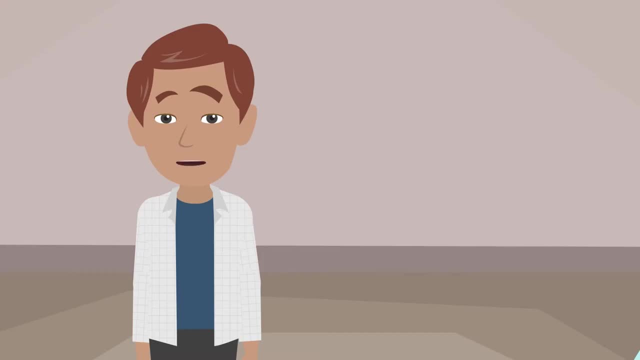 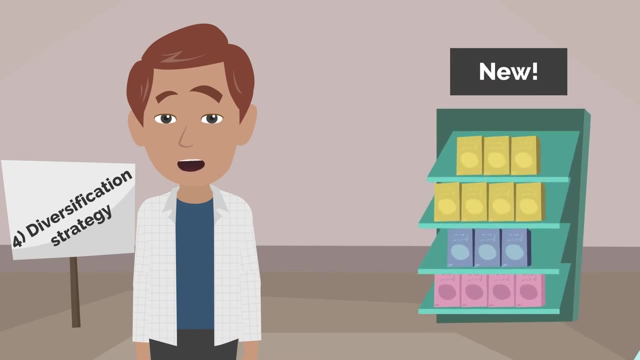 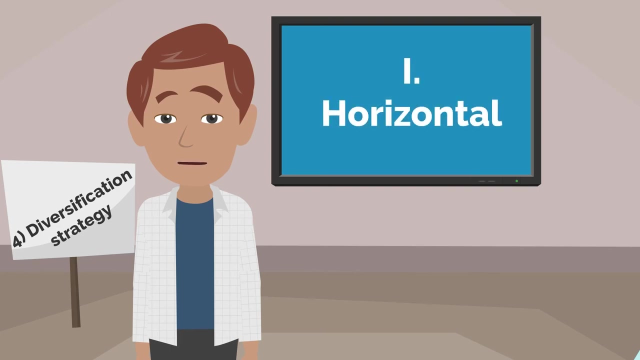 recipients. The last, most costly and time-consuming option is the Diversification strategy. It consists in offering products on new markets, resulting in the highest possible degree of expansion. There are three types of diversification: horizontal — developing new products for new markets with the help of the currently possessed technologies.